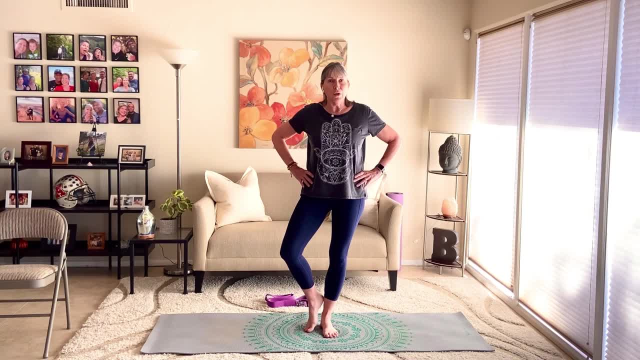 Pick up the right heel, Slide that right foot over until your right heel touches the left leg. You can stay there or you can pick up the right foot and bring it to the inner calf. If you bring it to the inner calf, press it together. Press the foot into the calf, the calf. 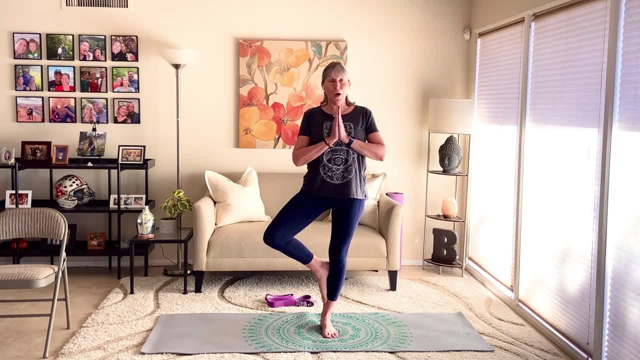 into the foot And we'll just bring the hands to the heart. Thumbs, palms together, thumbs at the heart, The standing leg getting a lot of good, strength and work. This femur, this hip, We're going to hold and breathe. Let that right knee open out to the right Good, And we're going to. 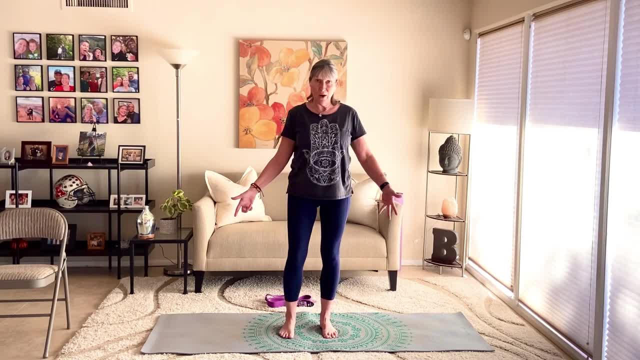 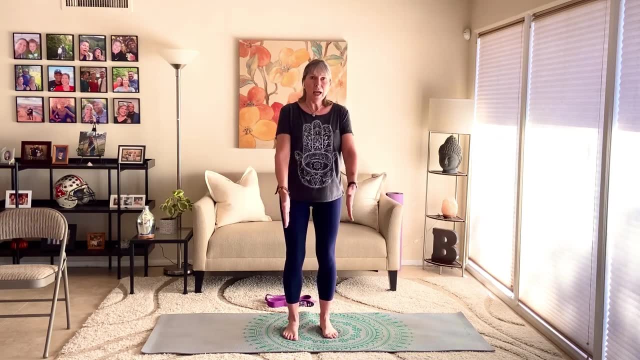 come out of it. Lower the hands, Bring your right foot down To the floor, Shake it out a little bit So you could always have a chair handy on that one side, if you like. Let's get that weight even back in both feet. Feet are hip width, apart From the 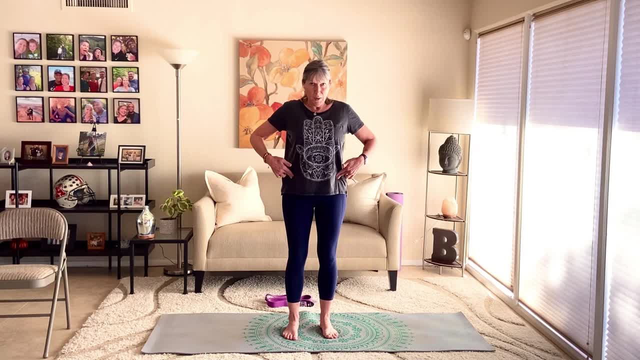 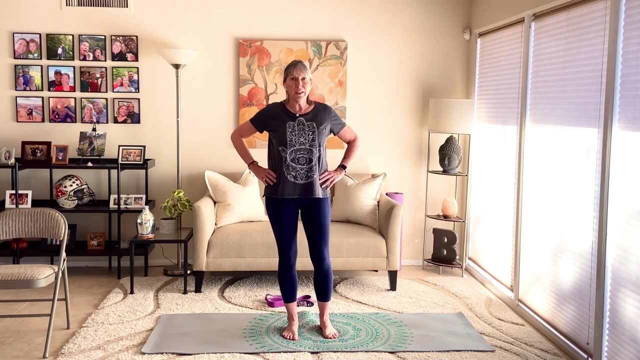 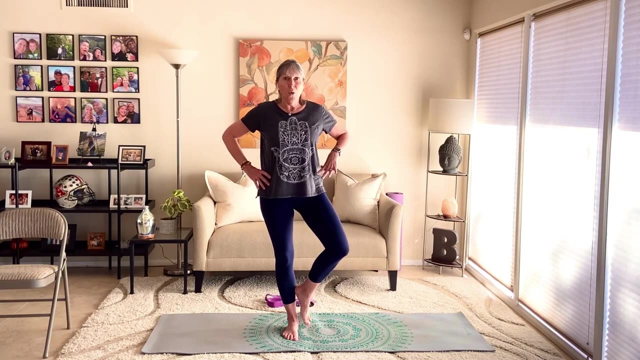 hip bones here, not the outer hips, but from where our hip bones are. we're going straight down. Start with hands on the hips. Shift all of your weight into the right foot. Lift the left heel, Slide that left foot over until it touches the right leg. You can stay there or pick up the left. 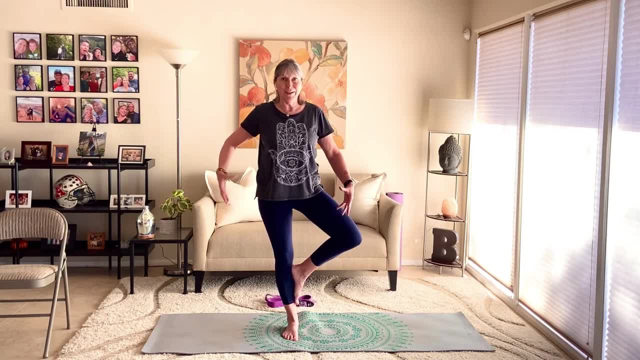 foot, Bring it to the right calf, Push the calf into the foot and the foot into the calf. Palms together, Thumbs at the heart. Belly pulls in and up a little bit. Lift the heart, Lift the chest. Little micro bend in that standing leg So we don't lock out the standing leg, knee, We're breathing. 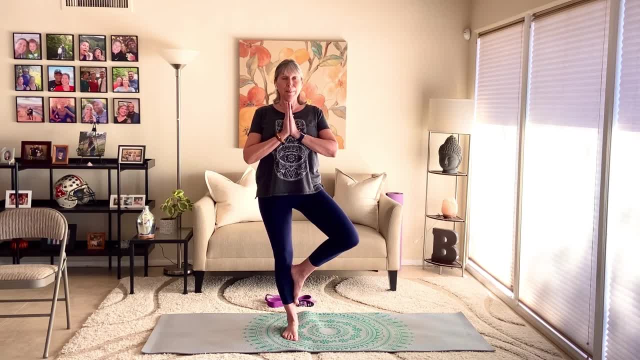 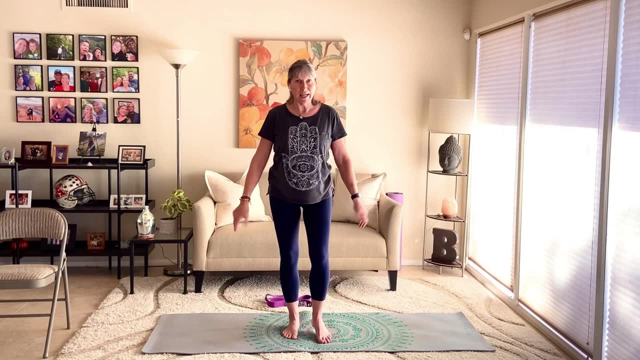 Building that strength now in the right leg, right femur, right hip. Good, We're going to come out of it. Bring the hands down, Bring the foot down and shake it out a little bit. So don't be afraid to do yoga poses Just. 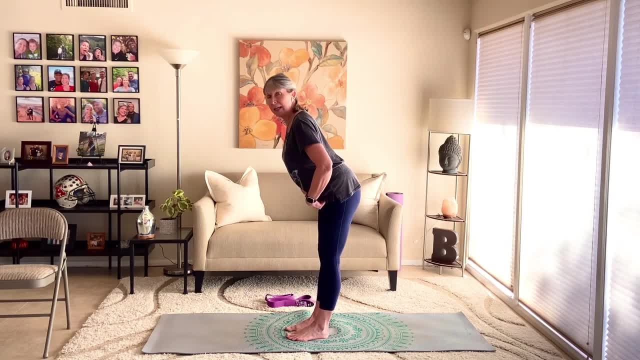 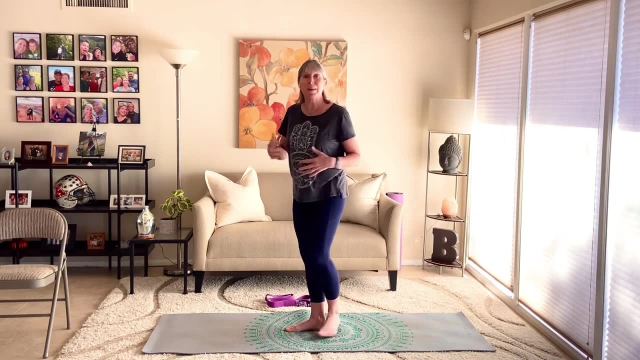 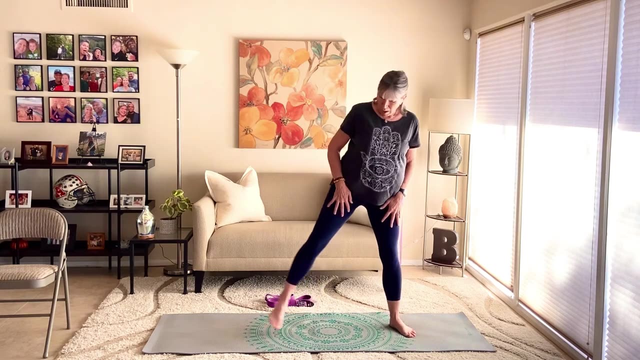 keep a nice long spine. We hinge at the hips, We don't round the spine. That puts a lot of weight and load on the spine And when you're twisting, twist with a nice long spine and don't overdo any of the poses. Number two pose of the 12 is triangle pose: Wide leg stance on your mat. 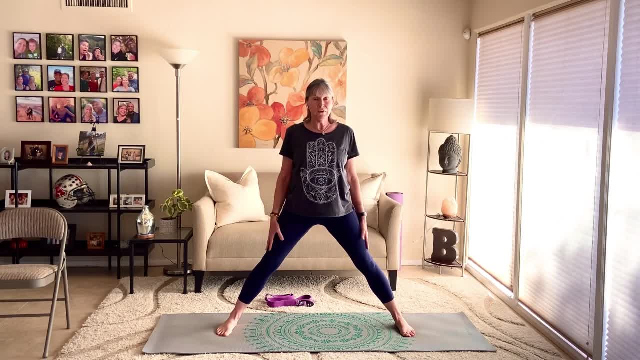 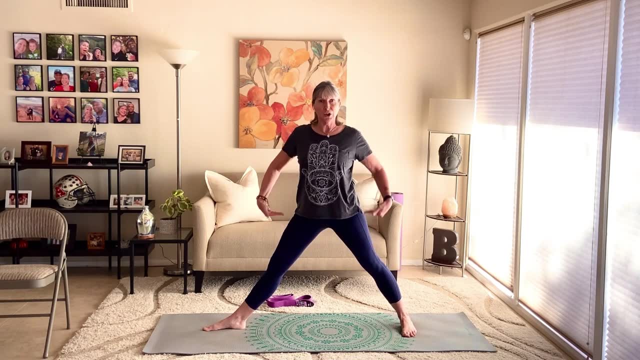 Your feet are three to three and a half feet apart. Keep your feet too close together. Right toes turn to the right, Left heel shifts back. Line up right heel, left arch. We're going to hinge from this hip, not from the waist. Inhale arms to shoulder. 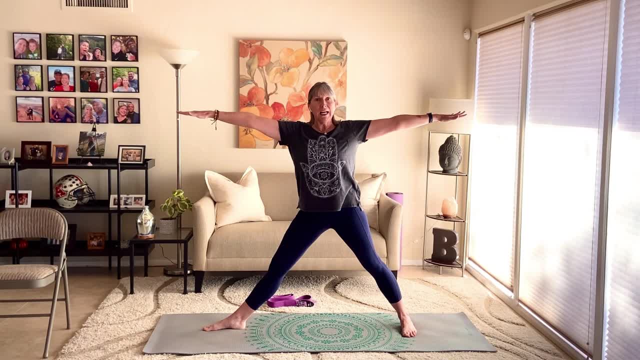 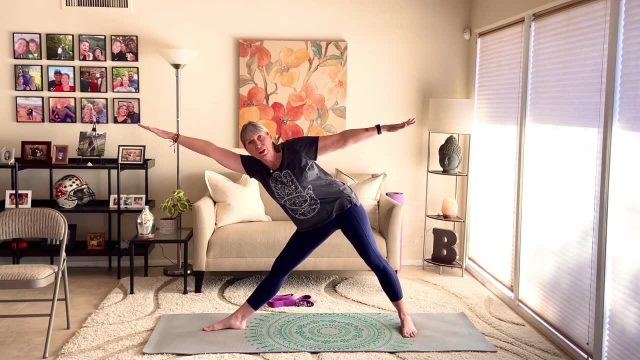 level. Exhale, Relax the shoulders, Inhale again, Exhale and hinge. Lean, lean, lean, lean to the right. Lean as far as you can. Keep your right rib cage long and then bring your right hand down to. 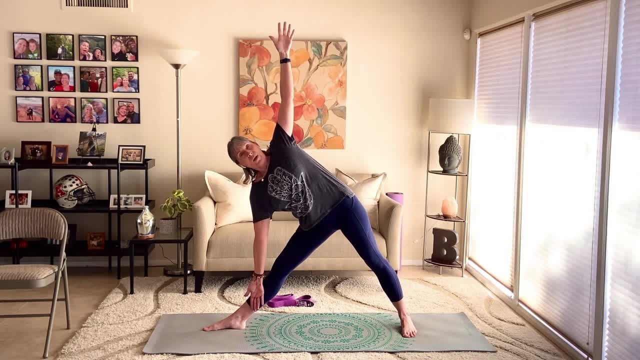 the right leg, Lift your left hand up, Pop shoulder back, Push the left foot into the floor. You're going to get a nice stretch on this inner right thigh. We're working the hips. The spine is long and straight. We're breathing Equal. 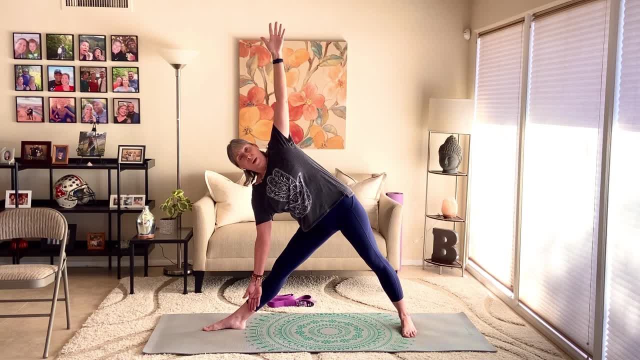 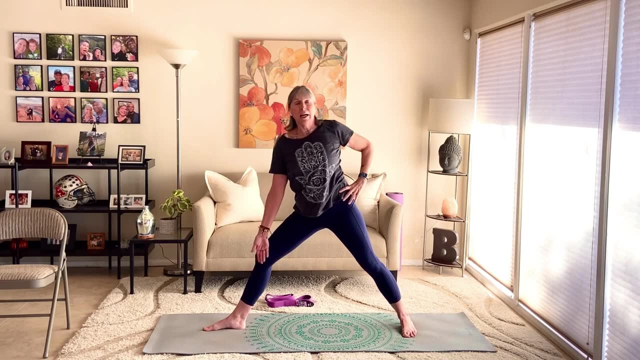 weight in your feet, in your legs. One more big breath, Let's come out of it. Bring the left hand to the left hip, Put a little bend in the right knee and inhale and come up. Straighten that right leg. Parallel the feet. Go the other way- Left toe. 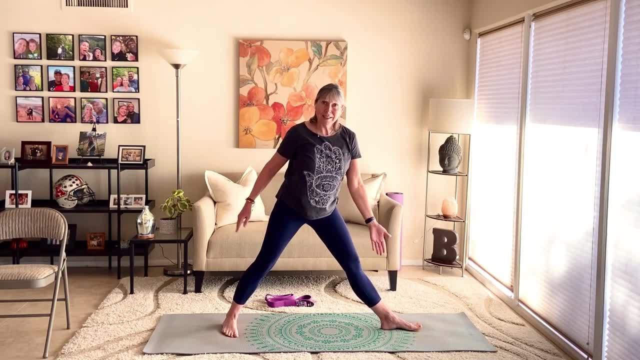 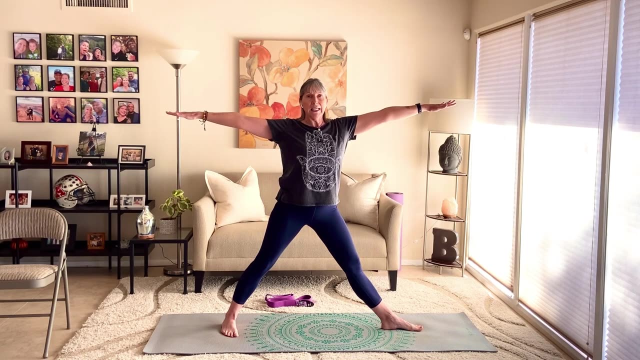 left leg. Left heel shifts back. Line up right heel. Left heel shifts back. Right heel shifts back. Set up your foundation. Left heel intersects right arch. We're going to hinge from this left hip, not from the waist. Inhale arms to shoulder level. Exhale. Relax the shoulders. Inhale again, Exhale. 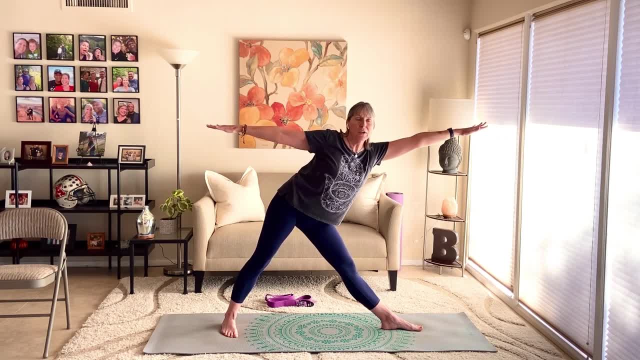 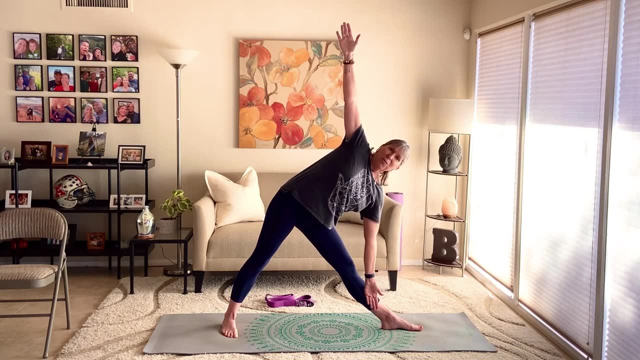 and lean Hinge. Reach to the left as far as you can. Keep that left rib cage long. Bring the left hand down, The right hand up. Keep the right foot pressed. Bring the left hand down The left hand up, Keep the right foot pressed. Bring the left hand down, The right hand up. Keep the right foot pressed. 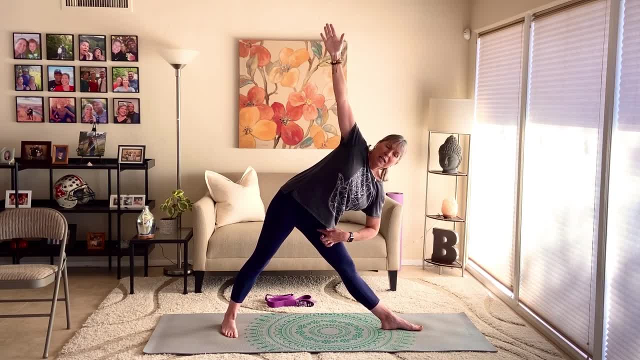 Pressing into the floor. This left rib cage is long, Getting a good stretch on this inner left thigh. Equal energy and weight in the feet, in the legs You're breathing. Top shoulder rolls back. Take one more nice inhale, One more exhale. Let's bring right hand to right hip. Put a little bend. 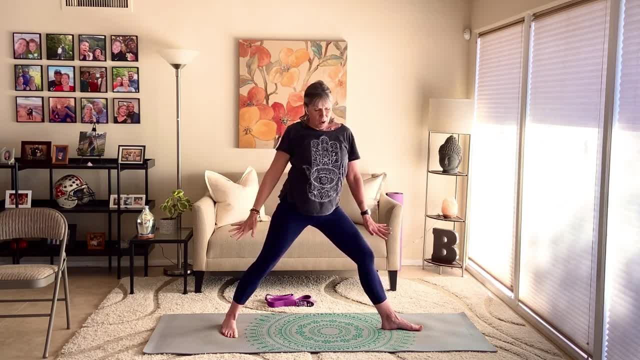 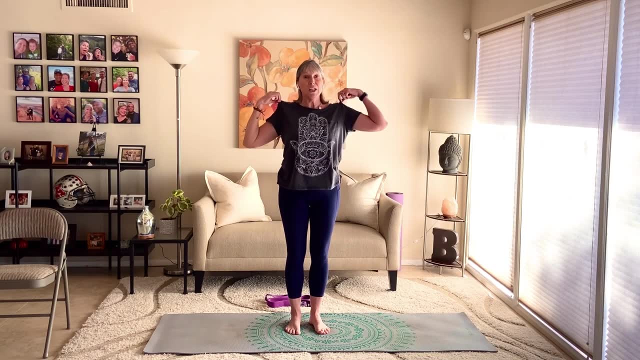 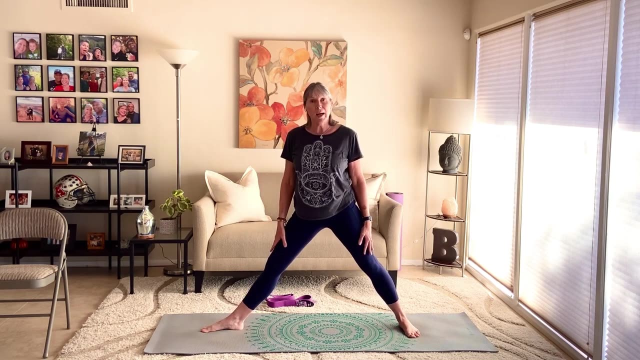 in the left knee and inhale: Come up, Drop the arms Parallel the feet. Good, Shake it out a bit. Number three pose is warrior two: Wide leg stance on your mat. Again, feet are three to three and a half feet apart. Right toes to the right. Left heel shifts back. We always line up right. 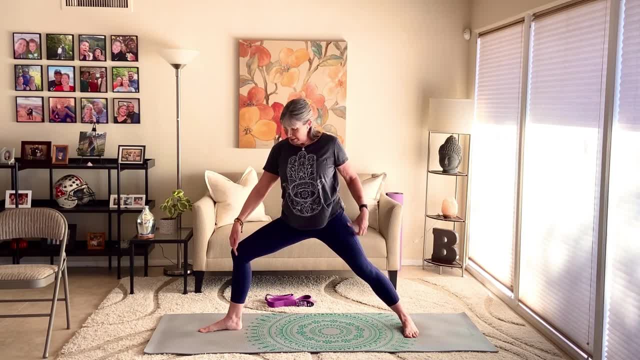 heel left arch. This time we bend the right knee. Right knee stacks over right heel Shoulders stack over hips. Right knee is going to open out to the right Inhale arms to shoulder level. Exhale, Relax the shoulders, Scoop that belly in and up. 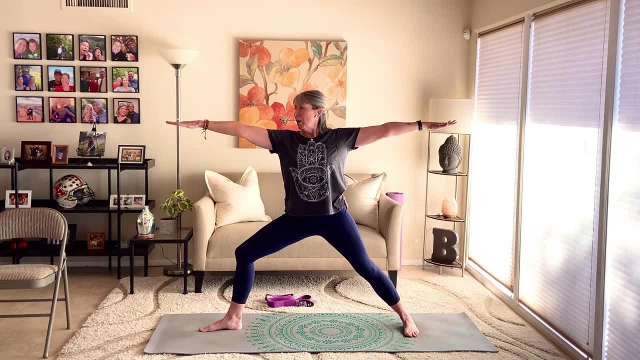 Look over the right fingertips. Equal weight, equal energy in the legs, the feet. The belly keeps pulling in and up Shoulders. relax down, Good, Strengthening the legs, the hips. We have a nice long spine. Let's lower the hands, Straighten the right leg, Parallel your feet. 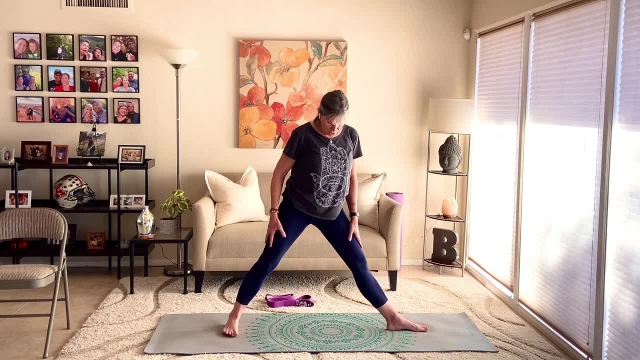 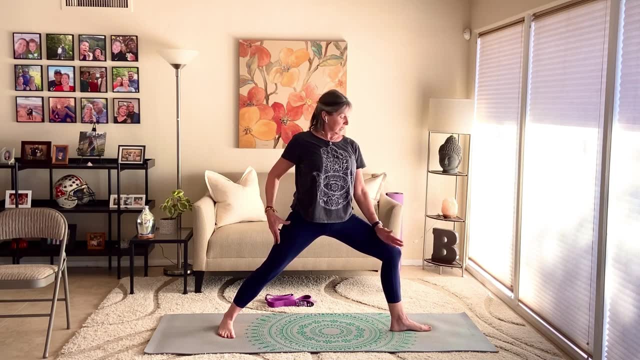 We're going to go to the other direction. Left toes turn to the left, Right heel shifts back. Line up left heel, right arch. Bend your left knee. Left knee stacks over the heel. Left knee opens out to the left a little bit. 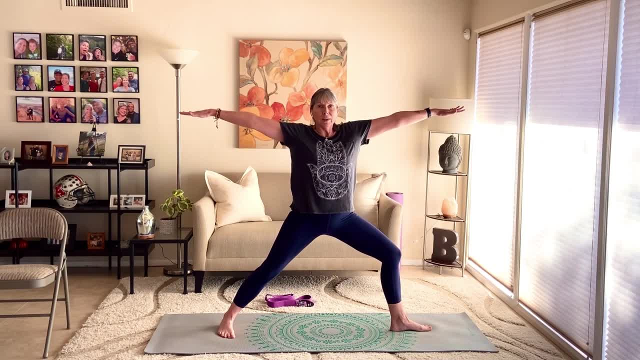 Shoulders. stack over the hips. Inhale. arms to shoulder level. Exhale. Relax the shoulders, Pull the belly in, Scoop it up, Turn and look over the left fingertips- Both feet pressing evenly equally into the floor. Work the legs When we press those feet into the floor. 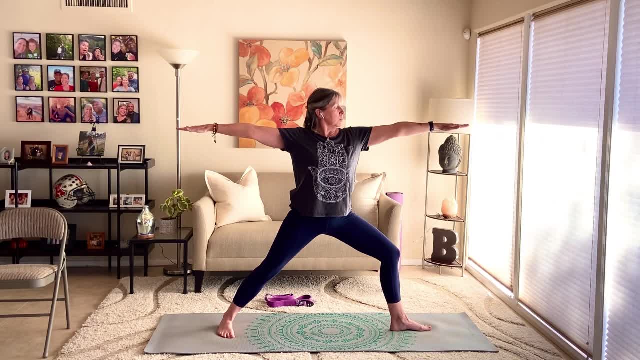 the muscles, hug the bones. Good Breathing. that right foot, right heel presses into the floor. Nice long spine. One more inhale, One more exhale. Let's lower the arms, Straighten the left knee, Parallel the feet, Step the feet together, Shake it out a little bit. 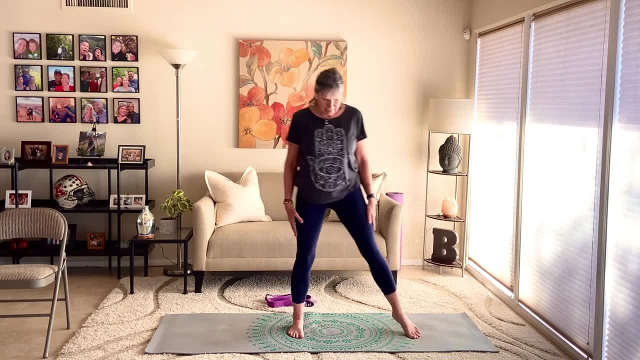 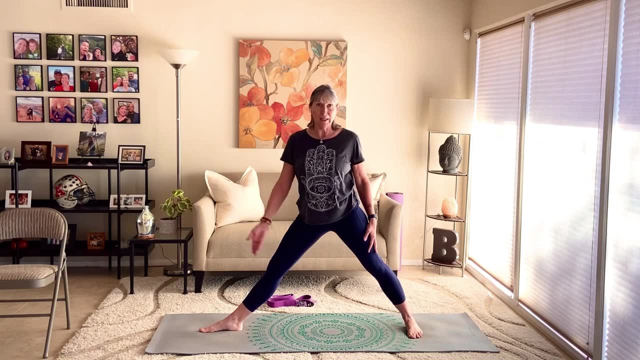 Beautiful. Number four pose: Extended side angle: Same wide leg stance. You get used to that, building that foundation. Right toes turn to the right, Left heel shifts back. We line that up. We're going to bend our right knee. It's going to stack over the right heel. 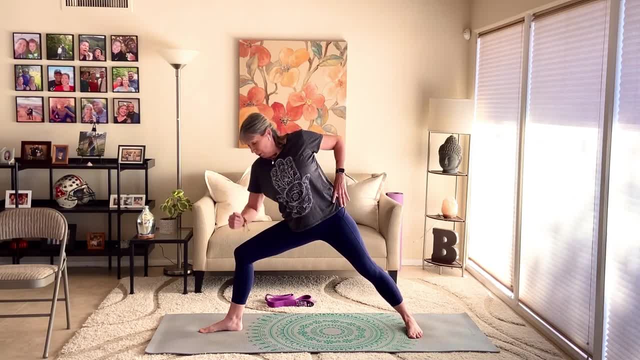 We're going to lean. hinge to the right. Bring your right forearm to the right thigh. Top shoulder rolls back, Left heel presses into the floor. Let's lift our left hand up and then bring that left arm by our left ear. Breathe Strong legs, Both feet pressing into the floor. 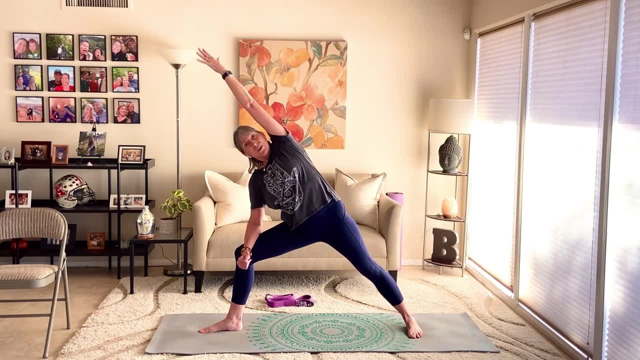 Really get that energy in the legs to work that right knee, Work the muscles to work And those muscles hug the bone to help build bone. Now, not too much weight here- Be able to lift up this right hand, right arm so that you're using your strong. 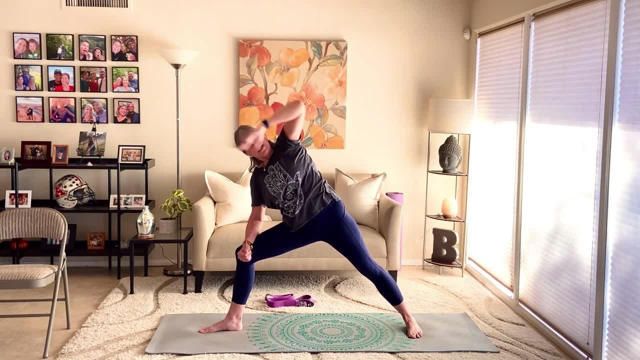 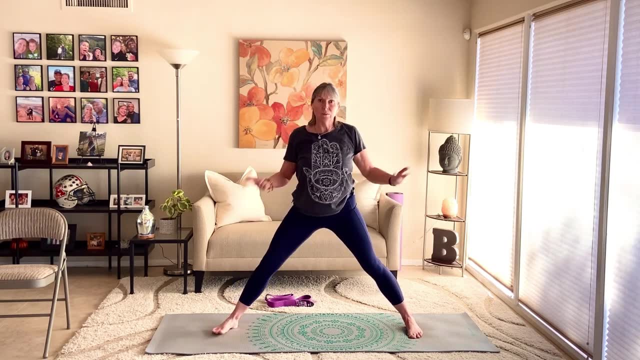 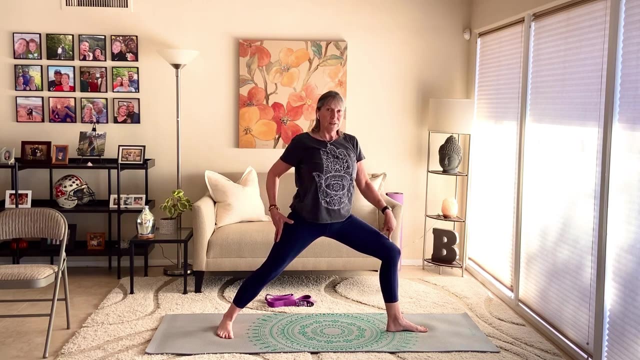 torso muscles. Let's come out of this pose. Bring the left hand to the left hip, Inhale. Come up, Straighten that right leg and parallel your feet. We're going to go the other way. Left toes turn to the left. Right heel shifts back. Bend your left knee, Left knee. 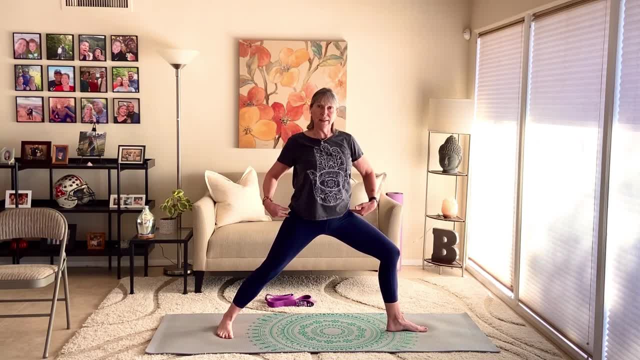 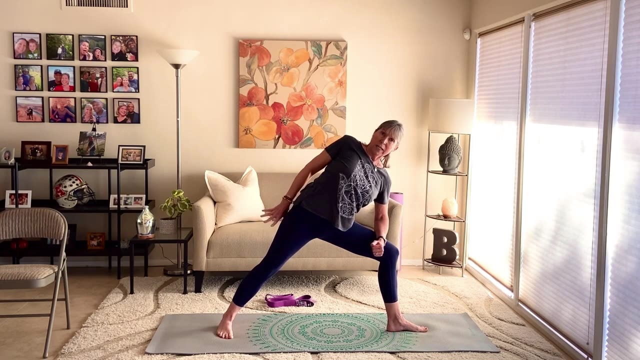 backs over left heel. We're going to hinge to the left, So inhale As you exhale, hinge to the left. My spine is nice and long. I'm bringing my left forearm to my left thigh, Right shoulder rolls back, My right heel pressing into the floor. Nice strength in both legs, Both feet pressing down. 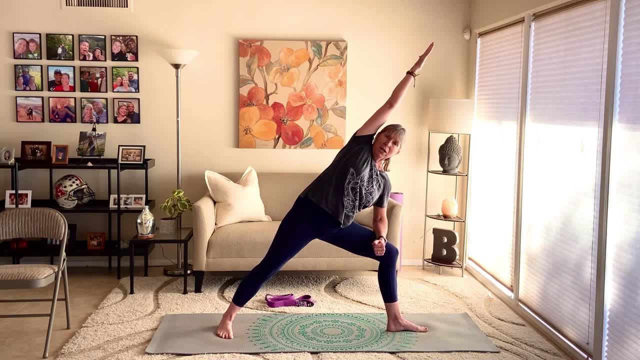 Stretch your right hand up and then bring your right arm by your right ear. Good Breathe here. Strengthen the legs, Lengthen the spine. Make sure you're not resting on that left leg. You should be able to lift up. 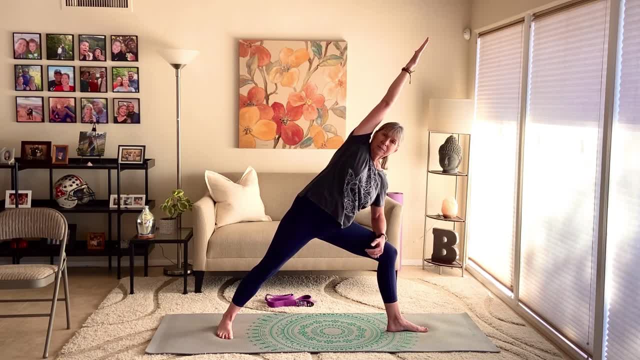 that left arm off of the leg. Let's take one more nice inhale and an exhale. We'll come out of it. Bring the right hand to the right hip. We're going to inhale and come up. Straighten that leg. 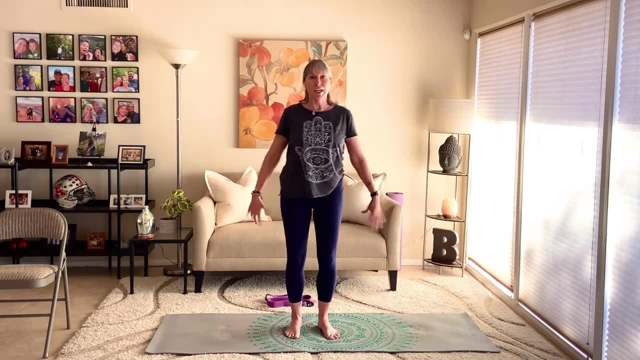 Parallel the feet. We'll step the feet together, Shake it out a little bit. Just shaking it out a little bit. Keep everything, even The body, even Number five is revolve triangle. So we're going to take that wide leg stance, just like we did. 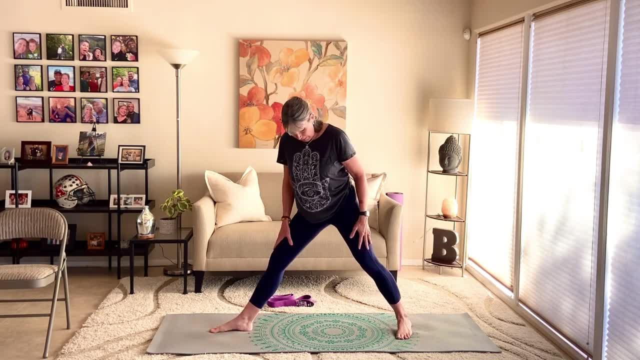 before, Turn your right toes to the right and your left heel back, like we did, But now I want you to walk that right foot just a little bit more to the right. So we've got a little space between our heels That's going to let us revolve our hips. So now we're going to turn our hips towards that. 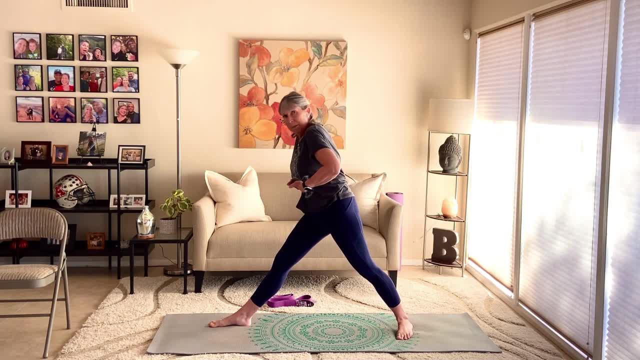 right foot. We keep a nice long spine. We don't bend from the waist. We're going to hinge from the hips. Inhale As you exhale, hinge forward. Long spine, You're going to bring the hands. Just start with the hands on that right thigh. Now bring your right hand to your right 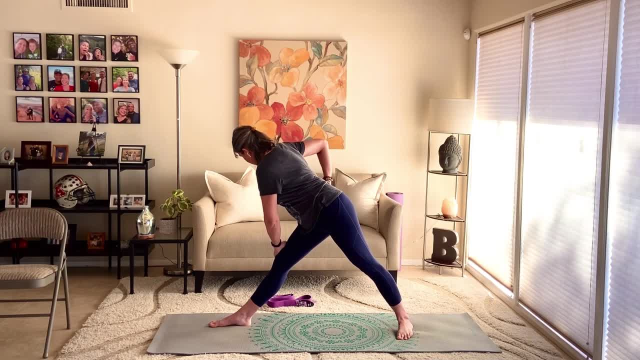 hip And we're pulling the right hip back And we're trying to turn towards the right. It's a revolved triangle, So don't worry, This is a tough pose, And so don't worry if you don't get too far. 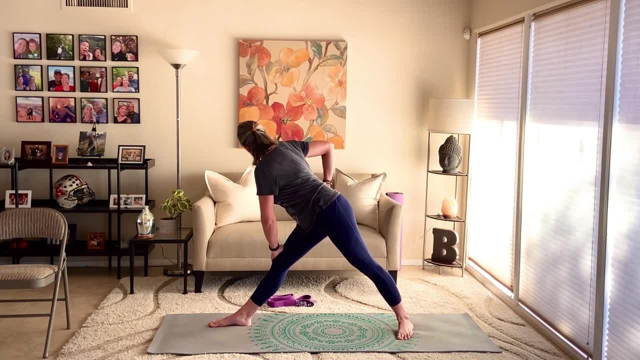 into it. But we're turning the hips so that the hips are facing forward And then we're going to lift that right arm up. It's okay if the right hand stays on the right hip, Totally fine To come out of it. turn your chest towards the floor. We're going to hinge up Nice long spine. We're. 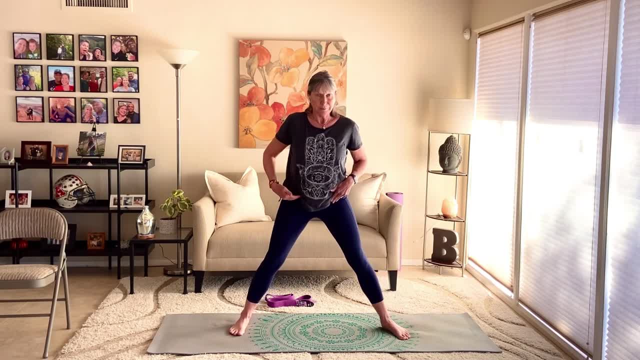 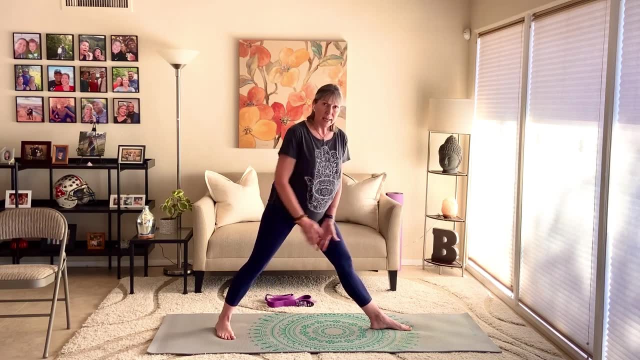 going to rotate forward And we're going to parallel the feet. Let's take it to the other side. Left toes turn to the left. Right heel shifts back. So we're still lining up that heel and arch, But now we're going to walk the left foot. 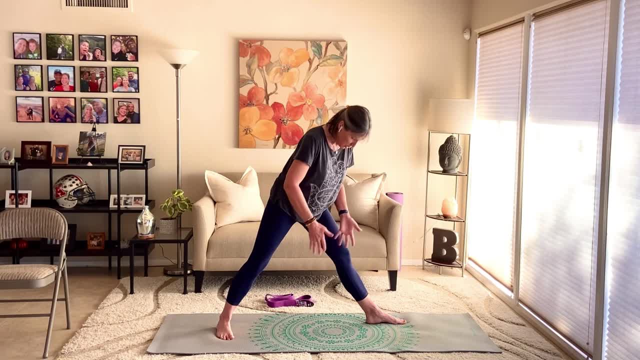 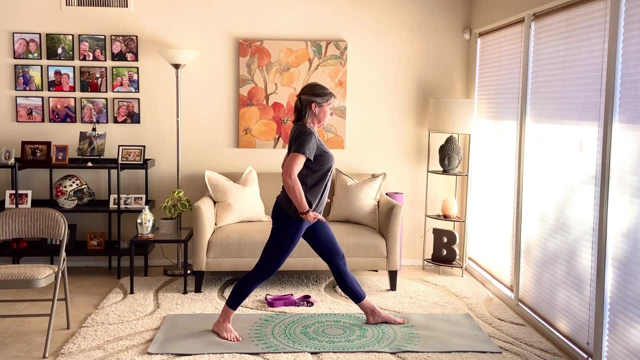 Just a little bit over towards the left edge of the mat. So we've got a little space between our heels. We're going to turn our hips towards that left foot. We're going to hinge forward from the hips. Inhale With your exhale. hinge forward, Long spine. Bring your hands to the left thigh. 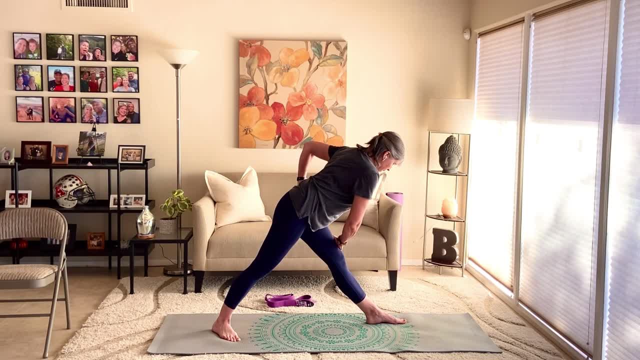 Now bring your left hand to the left hip And pull that left hip back And you're going to try to rotate Revolve to the left. Left hand can stay on the left hip, Or the left hand can stay on the right hip, Or the left hand can stretch up Breathe To come out of it. we're going to turn. 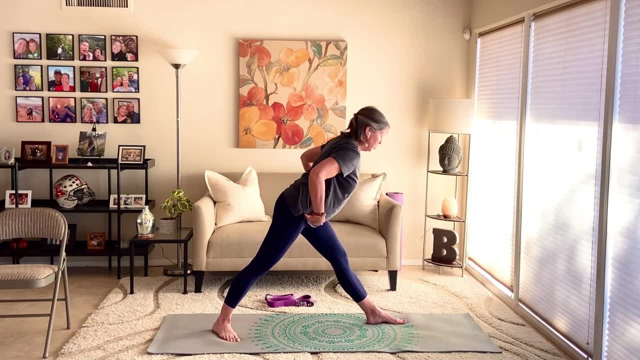 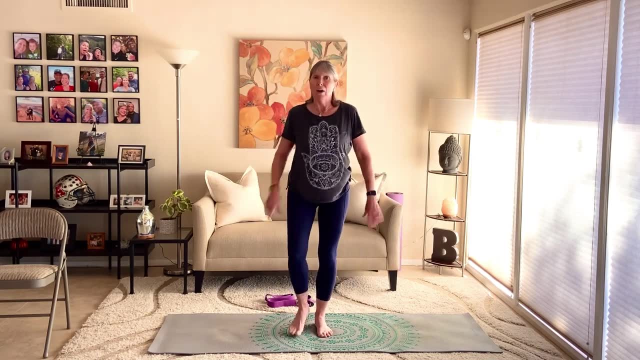 our chest back towards the floor. We're going to hinge up Parallel the feet And we're going to turn the feet forward. Step the feet together, Shake it out. That's a tough pose, So go little by little. You're getting the same benefit. if you just go in little increments, Don't worry. 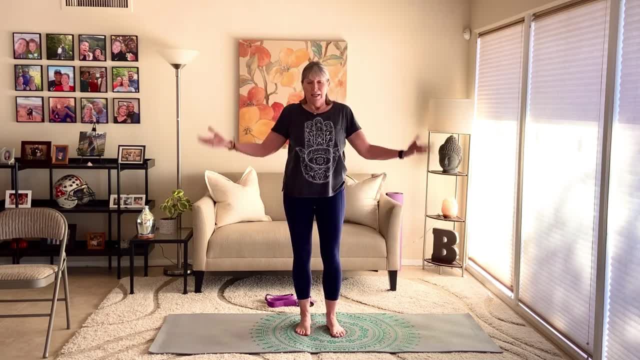 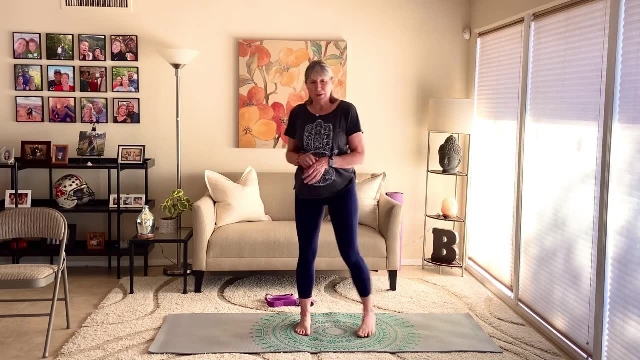 You're still going to get the same benefit if you're not in this fully calendar-worthy pose. The next one, we're coming down to the floor. We're going to come down to our belly Pose. number six is locust, So let's come down to the mat. Come on to your belly, Come down. 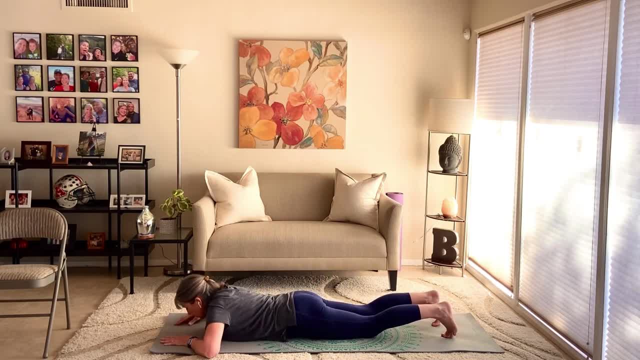 nice and slow. We're going to bring our arms down by our side, Palms are up, Foreheads on the mat. So our spine, our neck, nice and long, This is going to really work that upper back, upper spine. 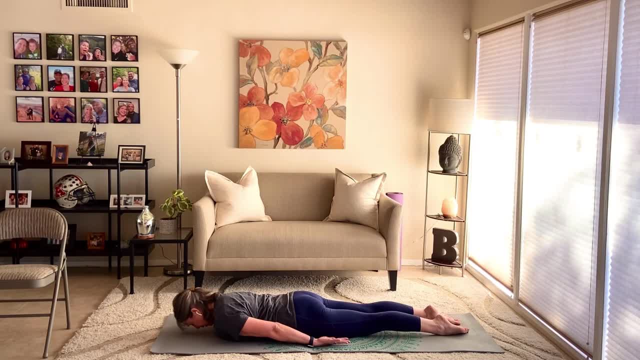 Firm up your legs, Firm up your body Bottom. So kind of squeeze the leg muscles, Squeeze the bottom muscles. We're going to lift our legs. Toes are pointed. Lift your arms. Squeeze your shoulder blades together And now lift your. 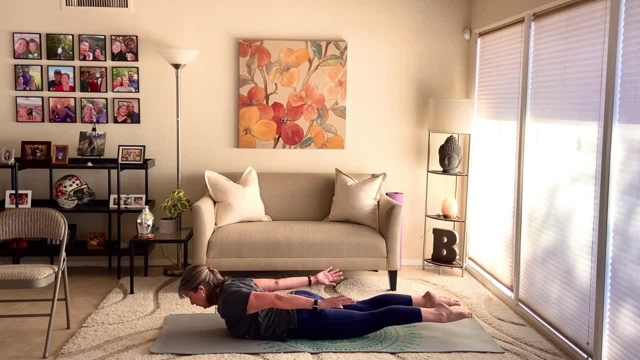 head and chest. The neck is long. Don't lift the chin too much. We don't want to pinch the back of the neck. We want a long neck, long spine. Squeeze those shoulder blades together. Keep the legs firm, bottom firm, Fingers reaching back. We're breathing into the belly. 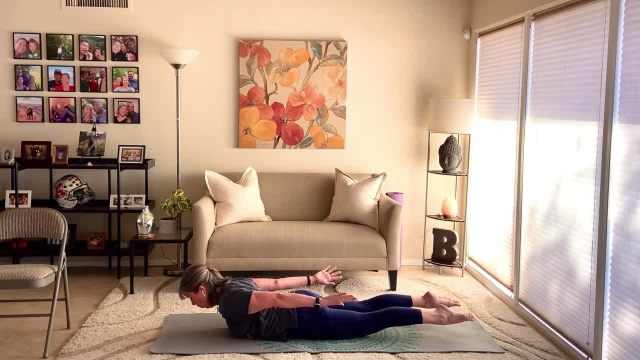 One more inhale, One more exhale And we're going to lower down. Stack your hands, Rest your forehead on stacked hands. Let the legs relax, Let your feet relax. Curl the toes under on the mat and push the heels back away from your knees. Lift off the mat. Just a stretch for your legs. 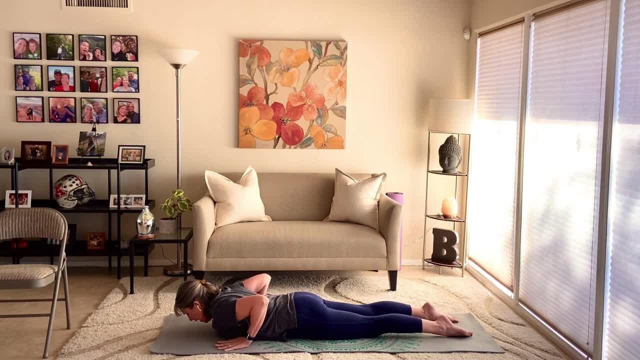 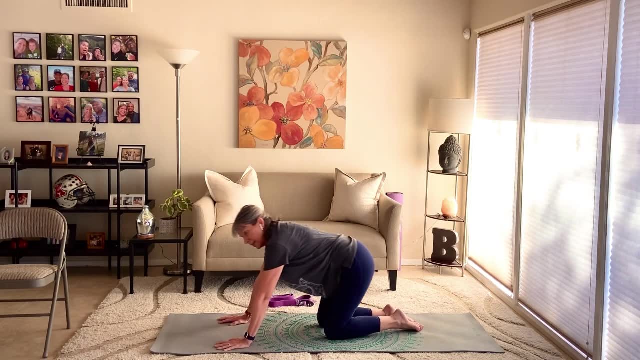 Relax the legs, Relax the feet And, nice and slow, Slide the hands under the shoulders, Lift yourself up into hands and knees. From table From table pose. we're going to sit back, We're going to swing our feet around, We're. 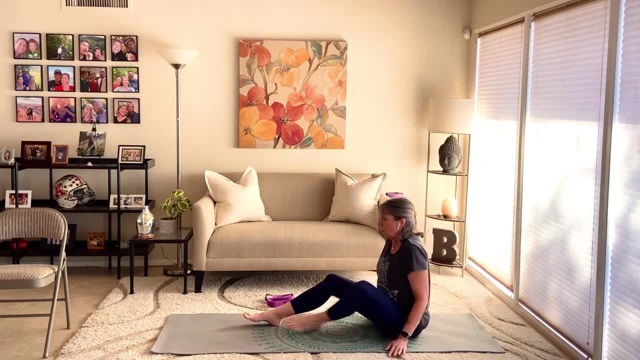 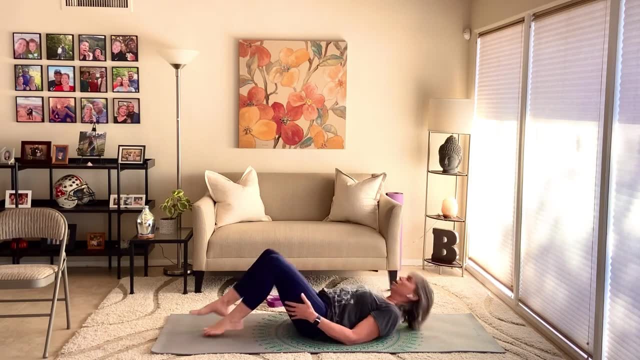 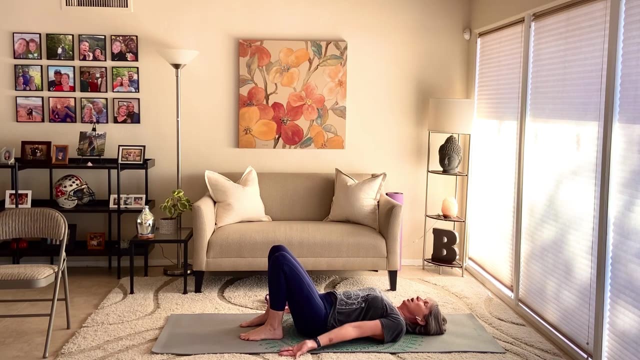 going to come down onto our back, Coming all the way down onto your back. for pose number seven is a bridge pose, So, lying down on your back, Knees are bent, Knees stacked over your heels, Feet are hip width apart, Arms at your side, Palms are up, We're going to lift our hips with breath Inhale first. 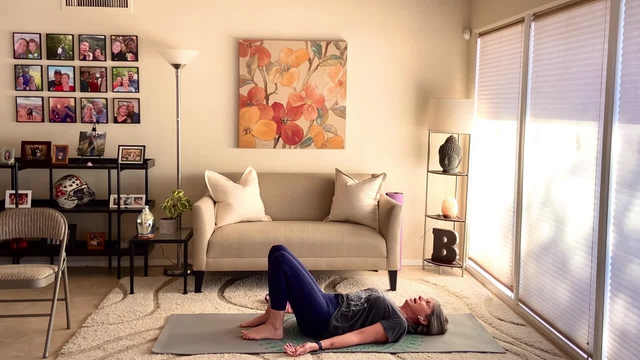 Exhale. Press your waistline down into the mat. Inhale, Lead with your tailbone and try to lift your spine up like a string of beads, One vertebra at a time. Go however high is comfortable. Walk the shoulder blades down and, under a little bit, Press the tops of the shoulders into the 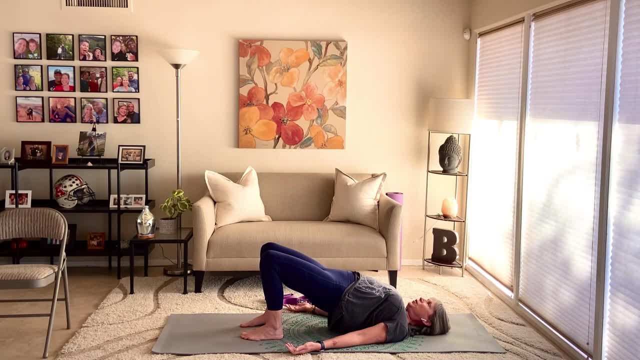 floor. Press the feet evenly equally into the floor. Belly soft, Bottom slightly firm. We'll take a few belly breaths here. So inhale Belly rises, Exhale, Belly falls. Keep pushing those feet into the floor. Keep sliding the knees away from the hips, Keep pressing your 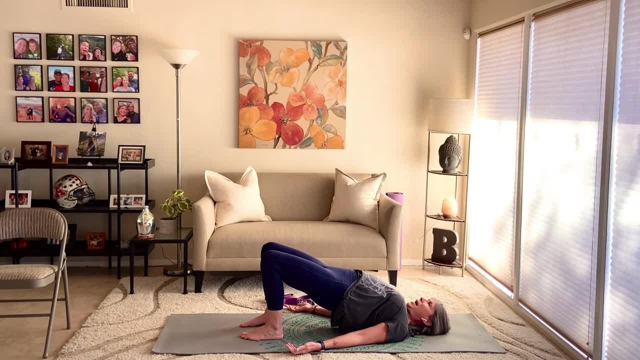 shoulders into the floor. Keep that spine nice and long. One more Inhale, One more Exhale. We're going lower with breath. Inhale with your exhale. Slide the shoulder blades apart. Lengthen spine. Try to set the spine down one vertebra there. 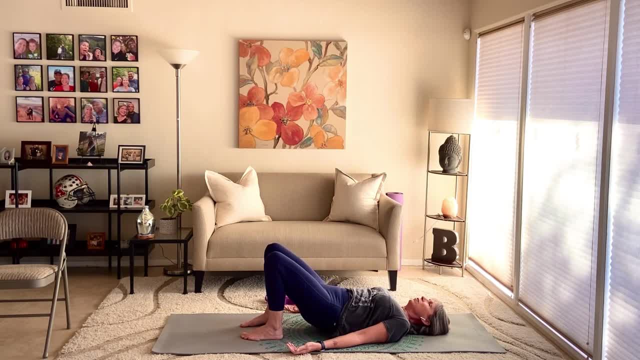 Come down in half a step, one vertebra at a time. Once your hips are down, hug the knees into the chest- Good work, And just roll side to side a couple times, Just rolling out that low back Knees to center. Use your core, Bring the feet down to the mat. 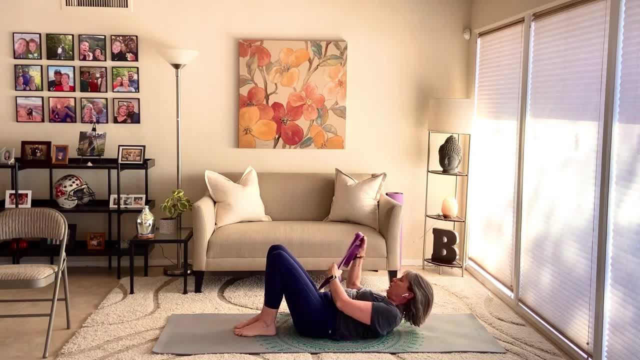 Here's where you're going to want that strap, So grab your strap. We're going to go into reclining big toe pose. We use a strap to help us. You can use a bathrobe tie if you don't have a yoga strap. We're going to take the strap and bring it around the bottom of the right foot. 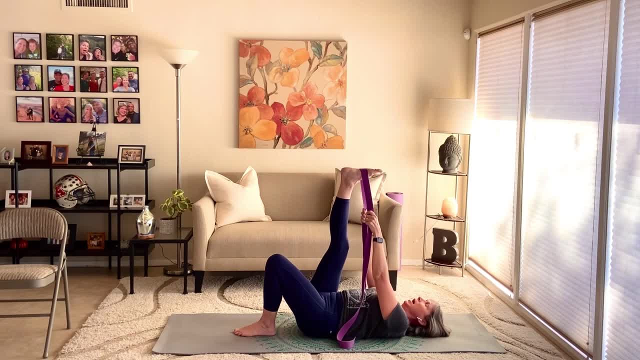 And we're going to stretch the right foot up to the sky. And here's where we're going to really strengthen this right leg, right hip, right femur. Try to lift and push your right foot up towards the ceiling And then, with both ends. 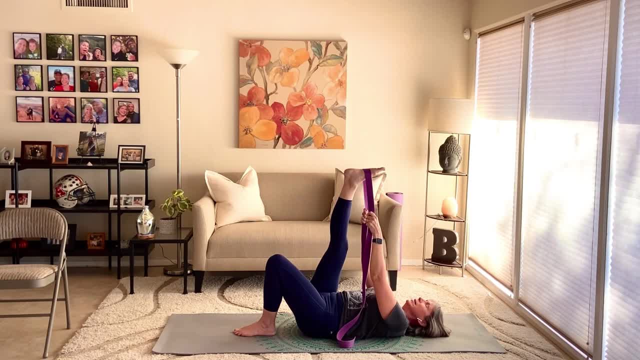 of the strap in both hands. we're going to pull the foot back down, So we want the foot and the strap to be opposing each other. The foot's trying to lift up and the strap is pulling the foot back down. So we feel that good energy and 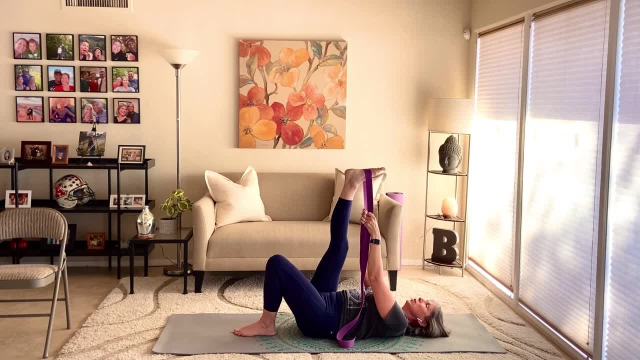 strength in that leg and the muscles in the hip. A couple more breaths. Spine is nice and flat and long on the floor. Good, We're going to come out of this. So bend your knee, We'll bring that right foot down. 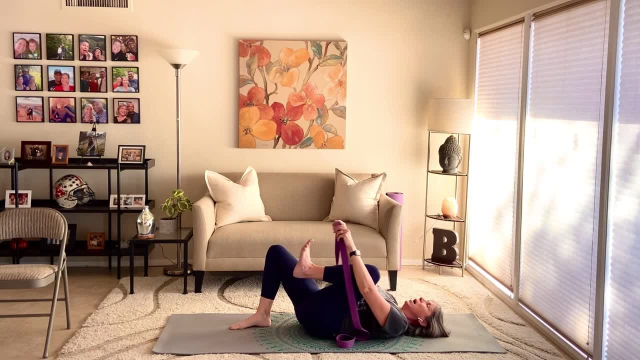 We're going to take the strap, wrap it around the bottom of the left foot. We'll stretch that left foot up to the sky, Hold each end of the strap in each hand. And now we want that isometric action. So the left foot pushing up towards the ceiling, but the strap pulling it. 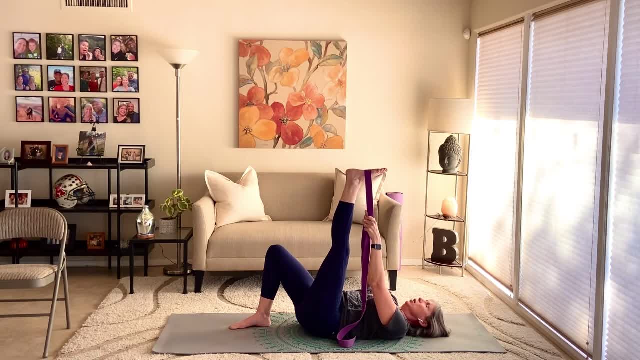 back down. They're opposing each other: That left foot trying to push away and the strap trying to pull it back down. So we're going to come out of this. So bend your knee, We'll bring it back down. That's what's really working. the muscles of the leg, Those muscles of the leg. 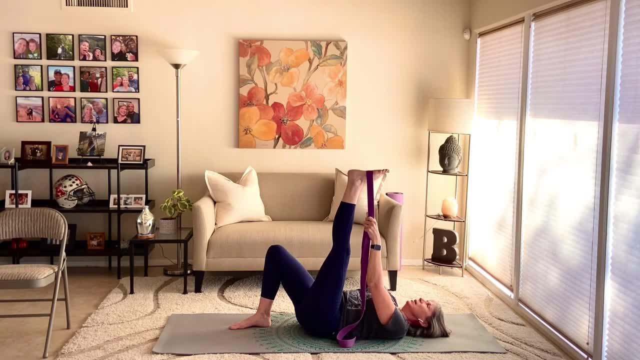 hug the bone, hug the hip and stimulate bone production. Nice, big breaths. Our spine is nice and long. You'll even feel strength in the arms here from holding on to the strap. One more inhale, One more exhale And then we're going to bend the knee and take that. 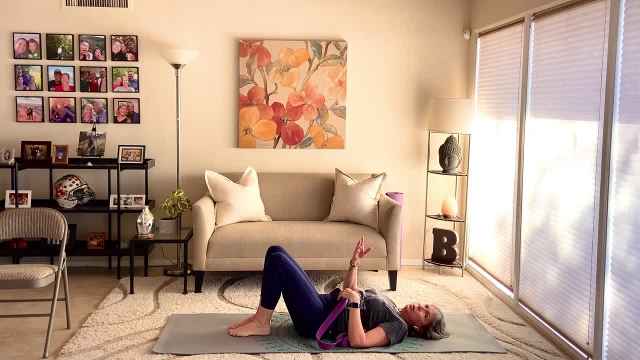 strap down. We're going to do that same pose with the strap around each foot, but we're going to open the leg out to the right. So let's take the strap on the bottom of the right foot again, Lift that right foot up to the sky. We're going to hold both ends of the strap in the right hand. 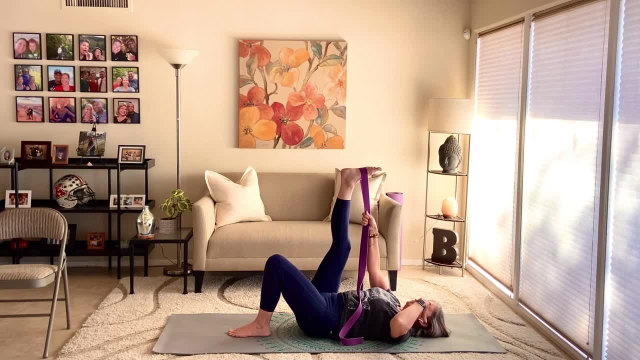 Left arm at your side, Left palm is up. We want to keep our back nice and flat on the floor and weight in the left side of the body. On your next inhale, open the leg out to the right Just a little bit, maybe halfway, Not too far. We want to keep that spine. 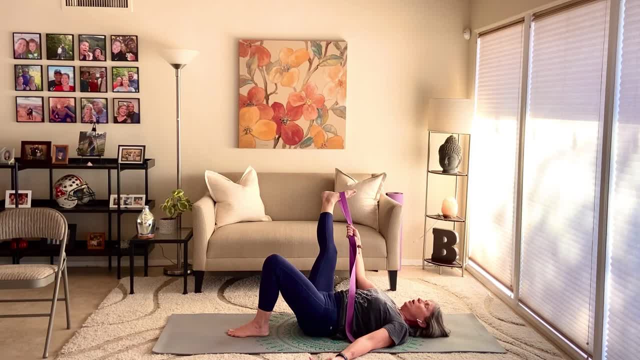 nice, and flat The left shoulder, left hip down on the floor. Now that same action of the right foot pressing away but the strap pulling it in. We want that action of that right leg. So try to push that right foot away from you, but pull the foot in with the strap. Nice, even steady belly breaths. 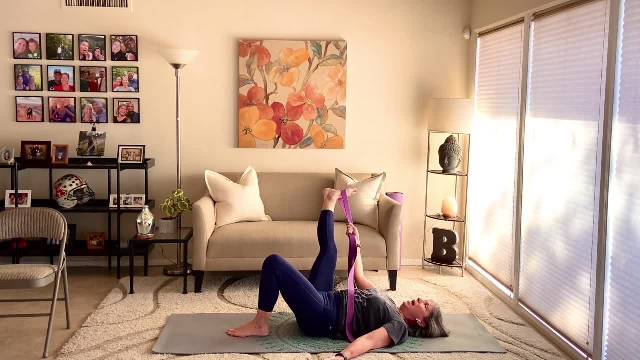 Good, Relax that action. Let's bring that right foot back up. Bend your right knee, Hug the right knee into the chest. Just let that the legs relax, that leg muscles relax. Bring your right foot down to the floor. We're going to switch the strap. Bring it on to the left foot, Stretch the left. 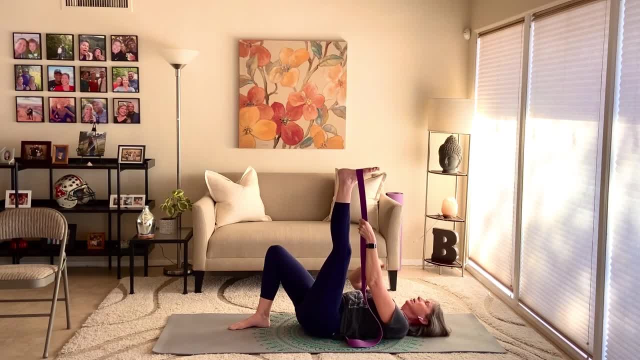 foot up to the sky. Hold both ends of the strap in the left hand Right arm at your side. Right palm is up. Keep weight in the right hand. Hold both ends of the strap in the left hand Right arm at the right arm, right shoulder, right hip. Keep your spine nice and flat And we're going to. 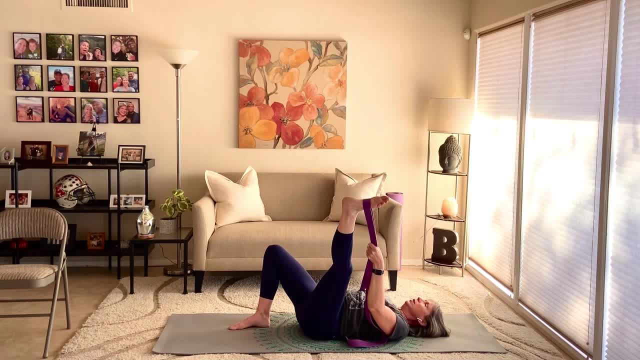 inhale, open the left leg out to the left. Just start with a little bit, but don't go more than halfway. Keep that weight in the right side Now push the left foot away from you and pull it in with the strap. So a lot of really isometric work here: the muscles, the energy opposing each 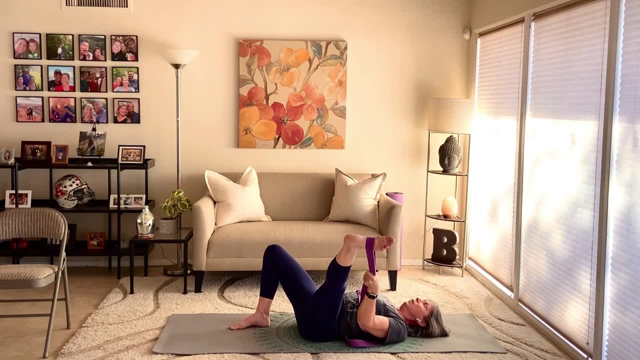 other Left foot pushing away strap. pulling the left foot in. Breathe into the belly- Inhale belly rises, Exhale, belly falls. Good work, Nice and slow. Let's bring that left foot back up. 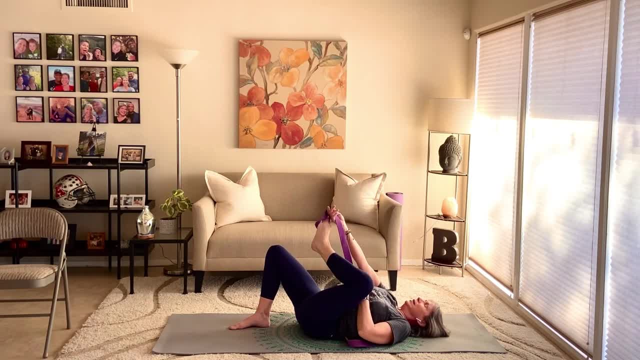 We're going to bend the left knee and bring that, hug that left knee in. You can set the strap aside. Let's just hug both knees into the chest here for a moment. Good, Use your core, Bring the feet down to the mat. We're going to roll to our side, either side. 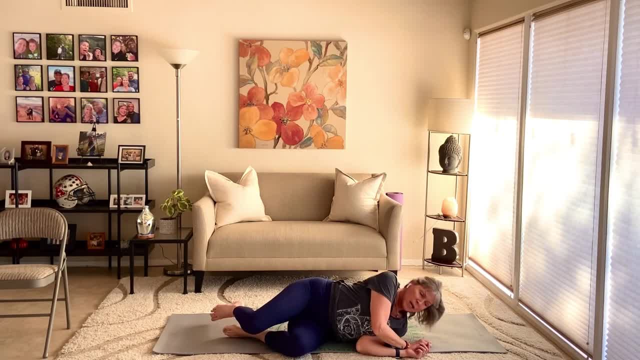 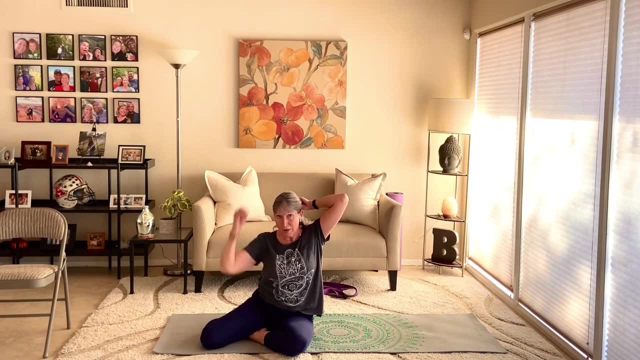 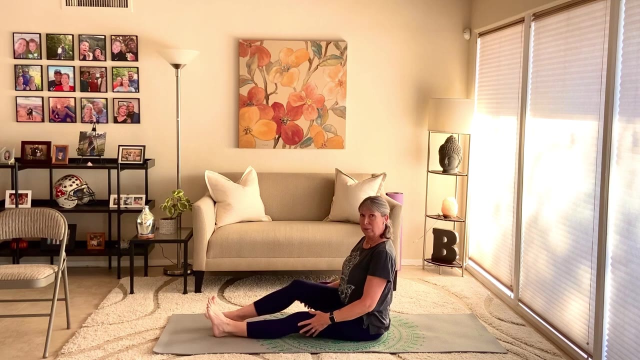 with a nice long spine. Use your arms to help you come all the way up to sitting. So the next one- number 10, is going to be a straight leg twist. So we're going to sit with the legs out. We're going to bend our right knee. Bring your right foot to the floor, Get the 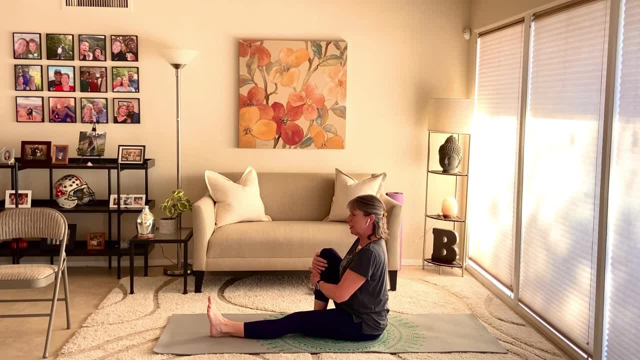 feet, even on both sitting bones. Left toes point up towards the ceiling, Left hand on the right knee, Right hand behind you or beside you. We always twist with an exhale. Keep your spine nice and long. Inhale, Press that right hand into the floor to lengthen your spine And with your exhale, 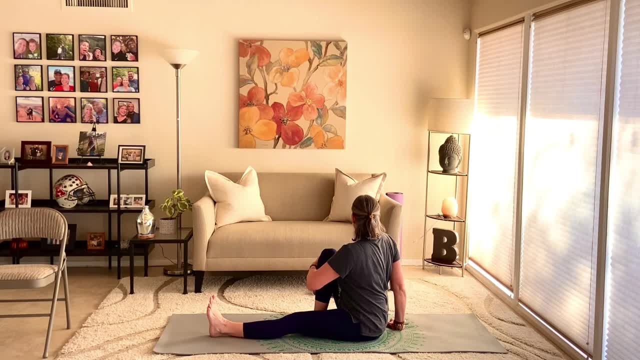 turn to the right. Hug the right thigh into the belly, Keep the spine nice and long Left toes pointing up The back of the left leg pressing into the floor. So we're turning. It's a nice, safe twist with a long spine And just go a little bit If it feels like you could go a little further. 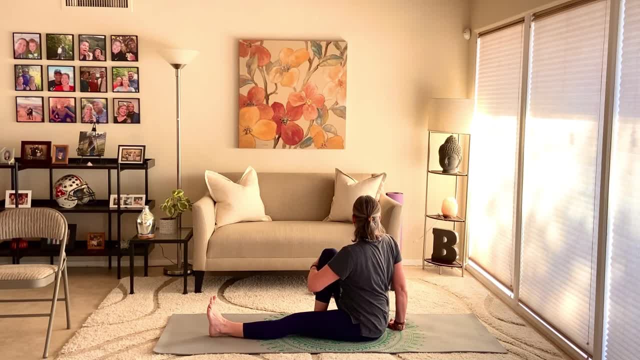 we don't overdo our twists when we're working with osteoporosis. We're breathing into the belly. We're going to come out of it, Inhale. Come forward, Stretch your right leg out. Bend your left knee, left foot. 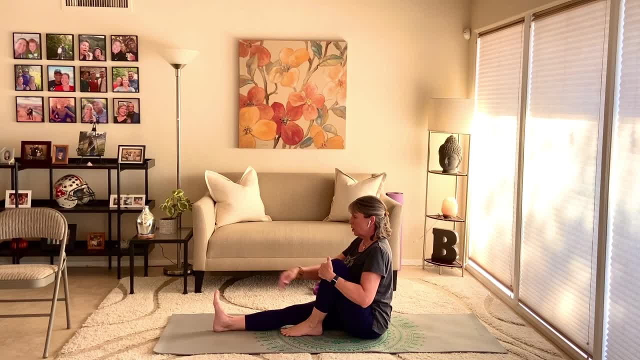 Get the weight even on both sitting bones: Right toes up towards the ceiling, Right hand on the left knee, Left hand behind you or beside you, Looking forward. we're going to inhale. Press the left hand into the floor to lengthen your spine And exhale. Turn to the left. Pull that left thigh. 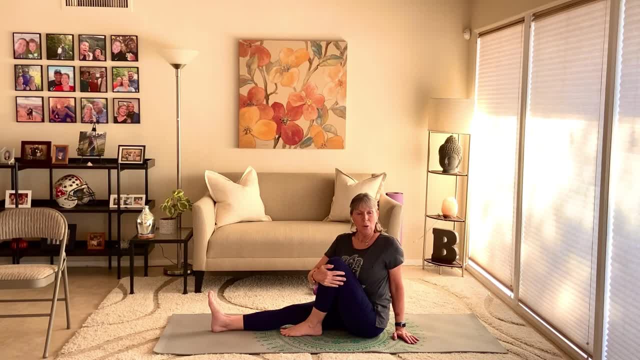 into the belly. Nice, slow belly breaths. We've got that weight even on both sitting bones. Nice, long, tall spine, The back of that right leg pressing into the floor, Right toes stay pointing straight up And we breathe into the low belly. We're going to come out of this. We're going to. 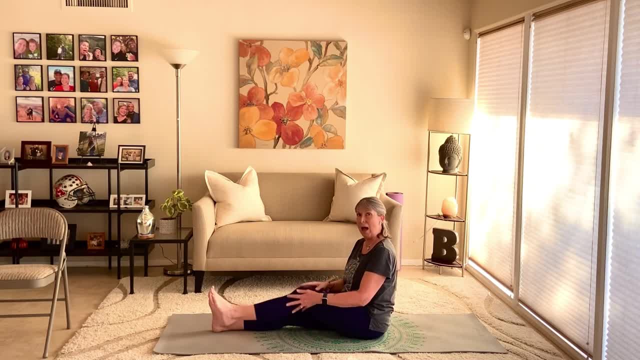 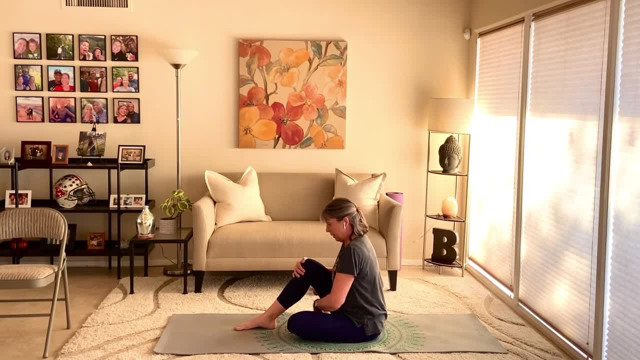 knees. We're going to bring our left heel underneath by our right hip. We're going to hug that right knee in, Get your weight even on both sitting bones: Left hand on the right knee, Right hand behind you or beside you. Remember we always twist with an exhale, So inhale, Press that right. 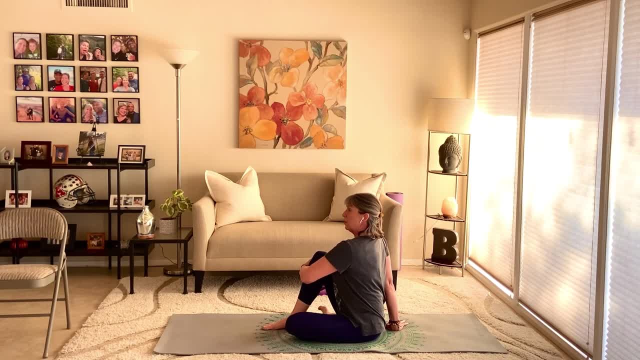 hand into the floor so you lengthen your spine With your exhale. turn to the right. Same as that last twist. We're pulling the right thigh into the belly. Our head is over the tailbone. We're not overdoing the twist, We're nice and gentle with it. 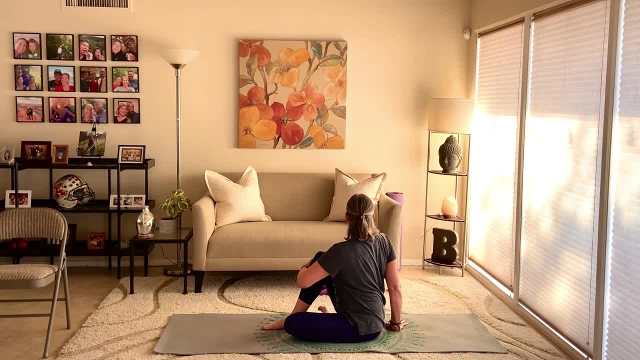 Twists are great for digestion, elimination, detox, getting all those toxins out of the body. Big breaths- So it's the big belly breaths that work here on the twists We're going to inhale to come out of it. 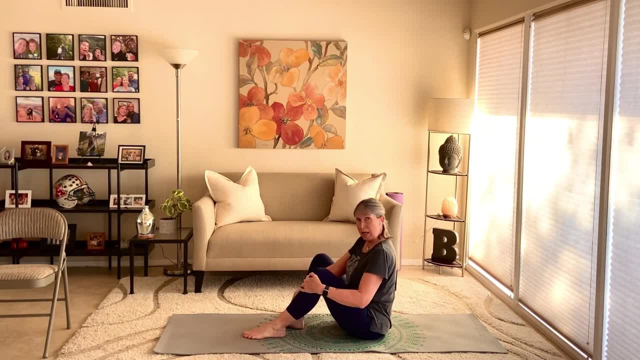 Bring the left foot out. Other side Right heel is going to come under by our left hip. We're going to pull that left foot in a little bit. Get your weight even on both sitting bones: Right hand on the left knee, Left hand behind you or beside you, Sit forward, Sit tall, Inhale, Press the left hand. 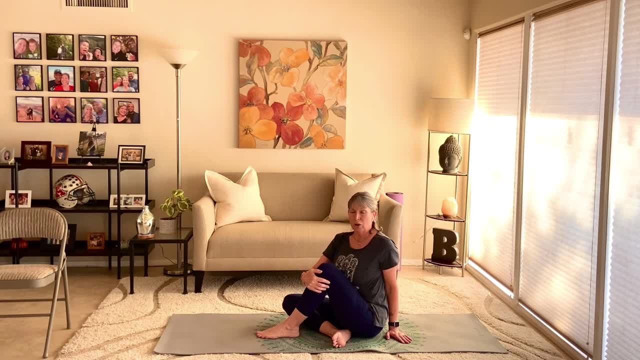 into the floor to lengthen the spine On your next exhale. turn to the left. We're going to pull that left thigh into the belly Head over the tailbone Spine. nice and long Weight even on those sitting bones. Just a nice gentle twist. Don't overdo it. 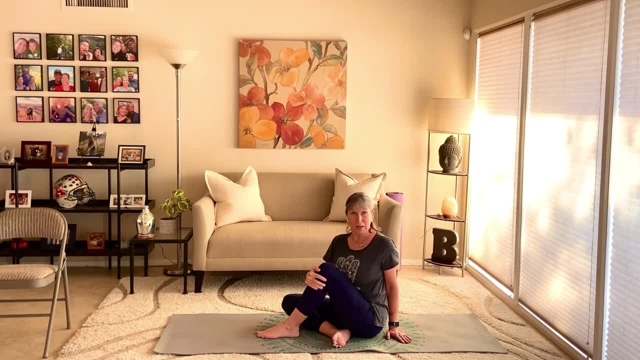 No need to overdo it. Your body's going to get all of the great benefits without over-efforting. The magic of twists is in the belly, is in that belly breathing When we inhale. that belly presses into that left thigh. It's working all those organs in the abdominal. 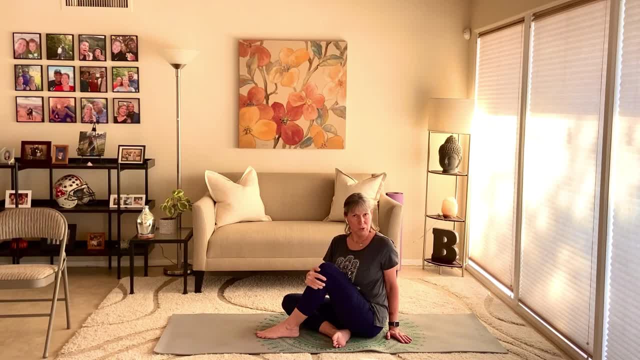 And we got this little torque on the spine, The hips, to increase that strength, Bone strength. We're going to come out of it. Inhale, Come forward. We'll bring that right foot out, One at a time. Stretch your legs out. 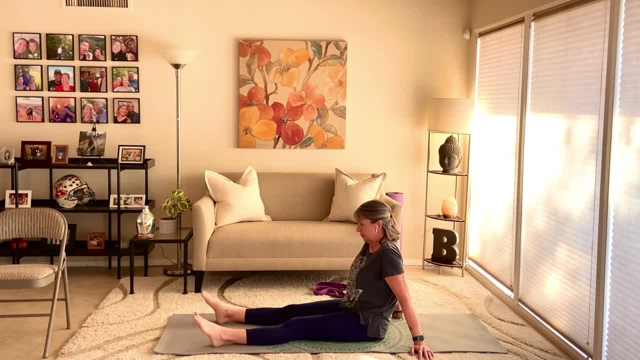 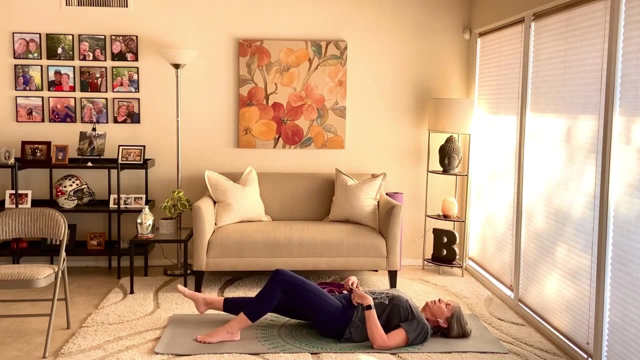 When she'll wipe her the feet. Just let the leg muscles relax And pose number 12.. Some people's favorite pose is Shavasana. So come down all the way down onto your back. Come down nice and slow, See if it feels good to keep the legs stretched out or maybe the knees bent, if you have any low. 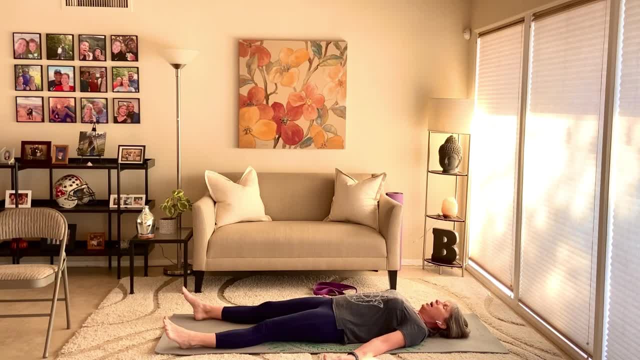 back pain, Knees bent is nice. Arms at your side, Palms up, Tuck the chin, Relax the shoulders. Start at the bottom of the feet and start scanning the body, relaxing each body part as you move slowly upward, all the way to the crown of the head. 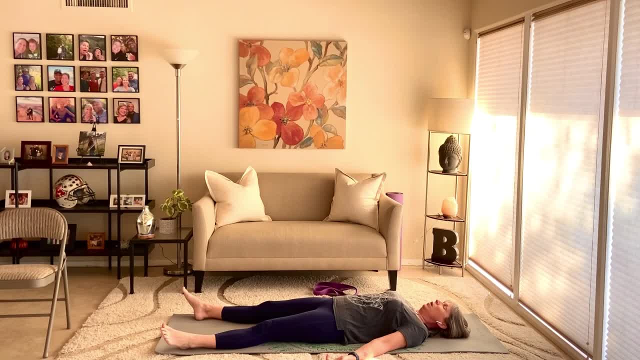 Make any little adjustments as you're moving your awareness from the bottom of the feet all the way up to the top of the head. Work on your belly, breathing. Inhale belly rises, Exhale belly falls. Our spine is nice and long. 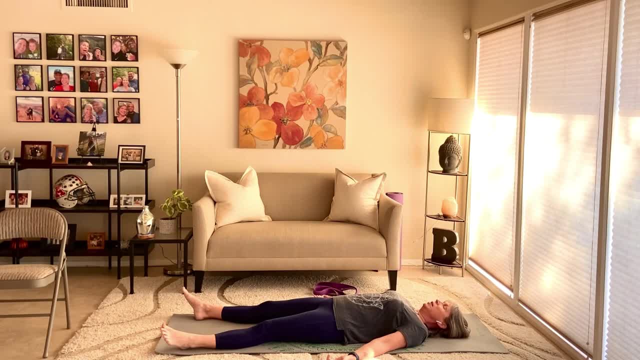 This final relaxation pose is where the body receives all of the benefits from a yoga practice: The stretching, the strengthening, the twisting. Now here I invite you to envision your bones strengthening, getting strong your muscles, strong your joints, mobile, flexible. 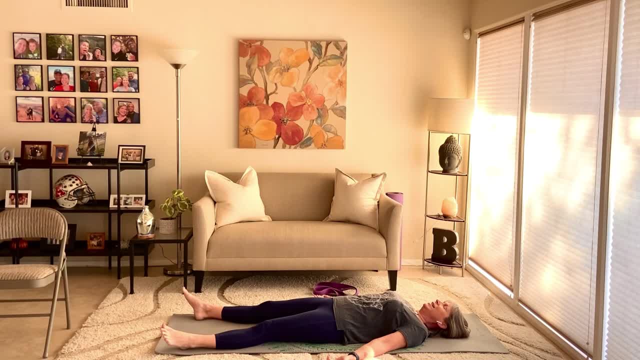 Inhale- Inhale health, vitality, strength, wellness. Exhale worry, concern, aches and pains. Use that visualization of inhaling strength and wellness and exhaling aches, pains, worries, concern With the body. 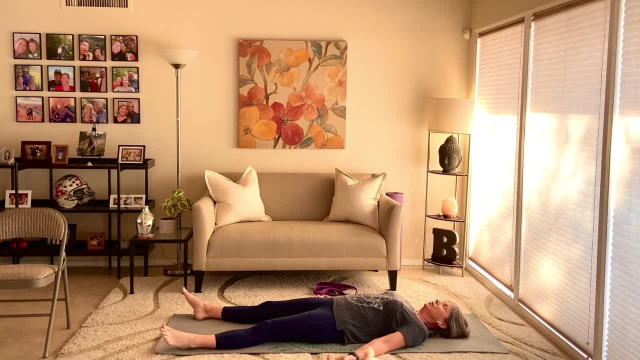 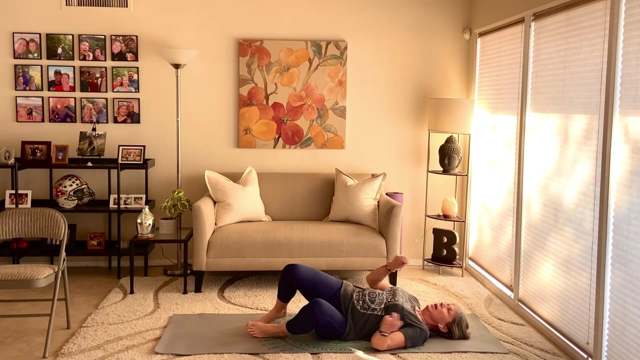 And completely relax. Let's wiggle the fingers, Wiggle the toes, Bend your knees, Bring your feet to the mat. We're going to come up to sitting, So roll to one side, Keep your spine nice and long, Use your arms to come all the way up to sitting. 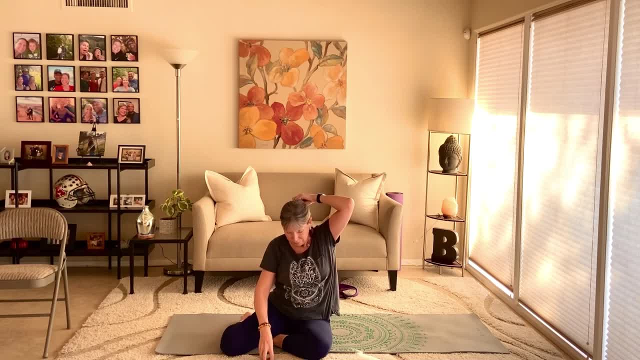 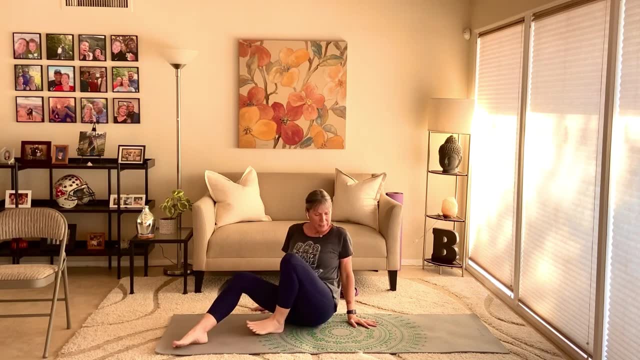 We're going to sit tall. We'll end our class. I like to sit on a yoga block, But wait, bring a yoga block out. Well, I'm not sitting on a yoga block then, But you're in your house, so you can sit on your couch. 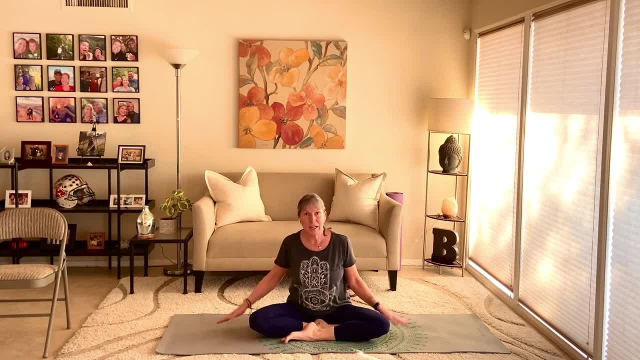 on a chair. sit cross-legged. You could be kneeling. You could bring have legs stretched out in front of you. We're going to sit with the shoulders over the hips, the head over the tailbone. Scoot the hips back a little bit. 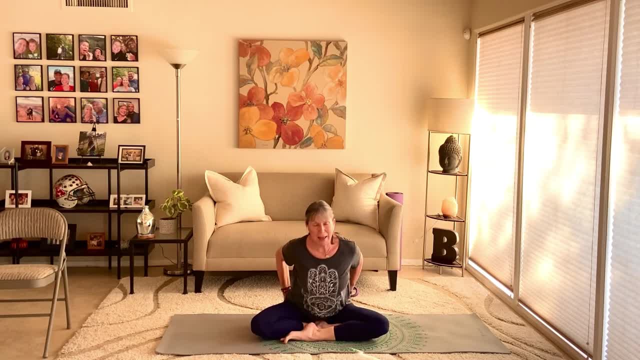 Lift the heart. bend the knees. We're going to sit with the shoulders over the hips, the head over the tailbone. Lift the heart. belly pulls in and up. Nice long spine. Let's bring the palms together. thumbs at the heart. 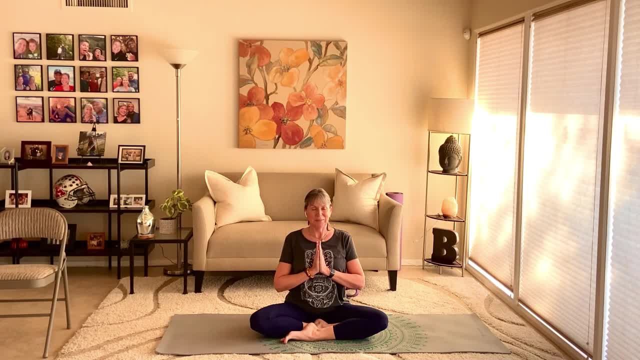 Symbolize ending sealing our practice today. Thank you for letting me share this with you, Namaste. I hope you enjoyed the practice. Check out some of my other videos. I've got yoga twists for osteoporosis, yoga for healthy joints.